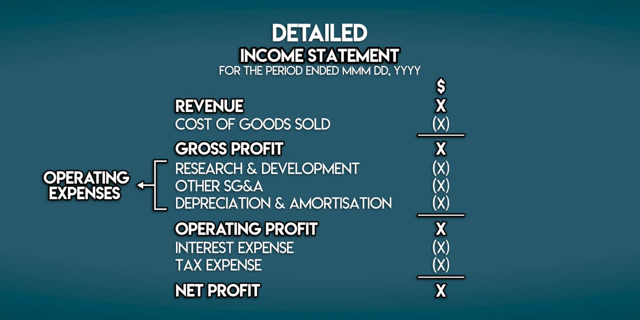 On the bottom line. we're left with net profit, which we'll get onto next time. so click subscribe if you'd like to watch that. You can find all of these videos in my financial ratios playlist, which I'll link to in the description. So one more time: what is operating? 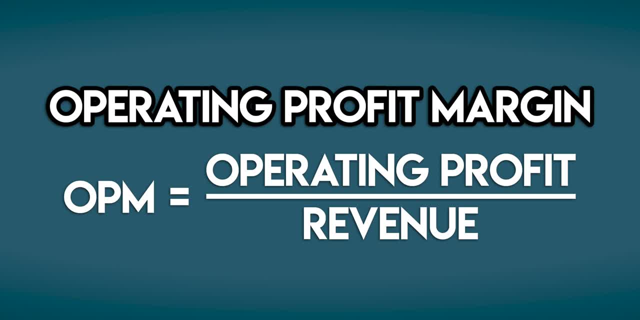 profit margin. Operating profit margin is a business's operating profit divided by its revenue And, by the way you can find this formula on my profitability ratios cheat sheet, which you can find in the description as well- It measures how much operating profit they're. 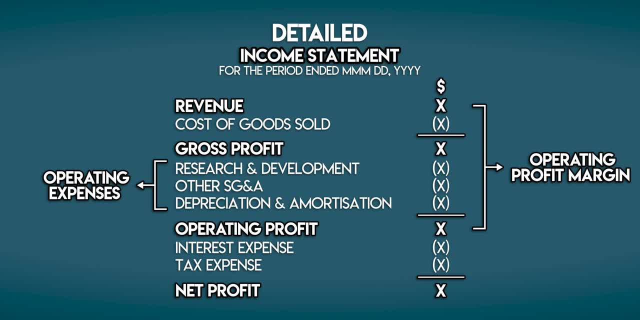 able to generate for each dollar of revenue earned. It only accounts for the business's direct cost of sales and operating expenses. It ignores the interest and tax expenses which we can see further down the income statement. Great, so let's do an example. 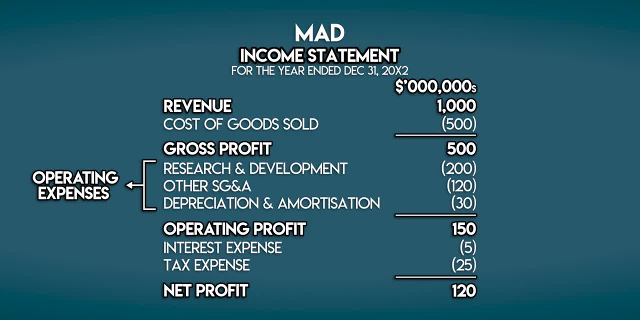 Here's the income statement for a business called ML, A tech company that makes semiconductor products. It summarizes the revenue they earned and the expenses they incurred over a one-year period. But what is MAD's operating profit margin? Well, we can see that they earned revenue of $1 billion and, after subtracting their cost of sales, 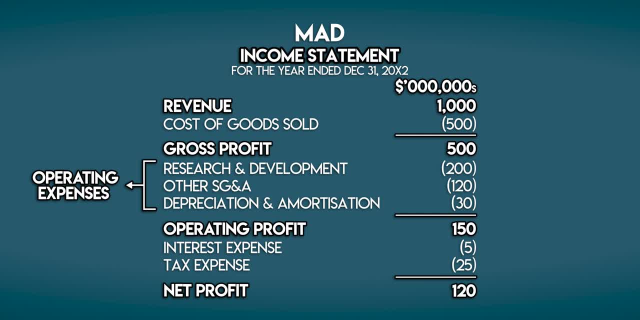 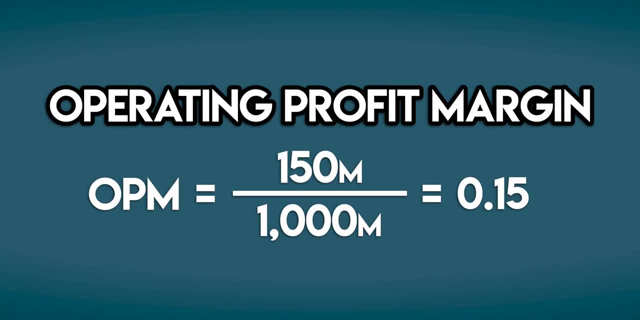 and operating expenses, they were left with an operating profit of $150 million. So their operating profit margin is $150 million. And after subtracting their cost of sales and operating expenses, they were left with an operating profit of $150 million. So their operating profit margin is $150 million in operating profit divided by $1 billion in revenue. 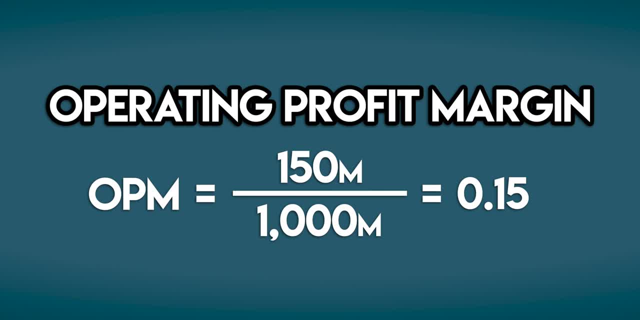 That's 15 cents of operating profit generated for each dollar earned, or 15% when we times it by 100.. Very nice, But whilst it's helpful for us to know this number, operating profit margin becomes more valuable when we make comparisons. For example, we can compare it year on year. 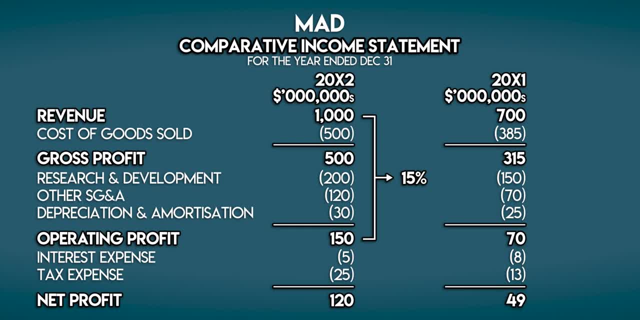 and we can see that MAD's income statement is $150 million in operating profit. Here are MAD's income statements for the past two years. In the current year they generated $150 million in operating profit, with an operating margin of 15%. 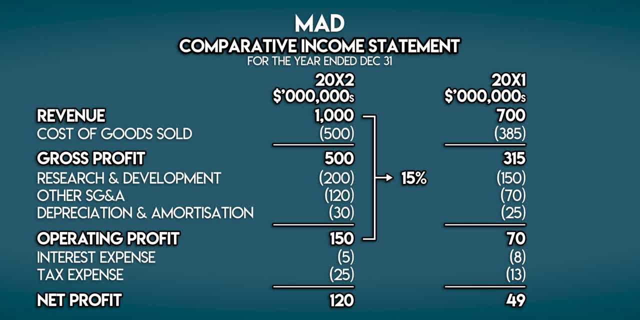 But in the previous year they only managed an operating profit of $70 million. When we divide that by their revenue of $700 million, we can see that their operating profit margin was 10%. So overall that's a 5% increase in operating profit margin year-on-year, Which is not bad at all. 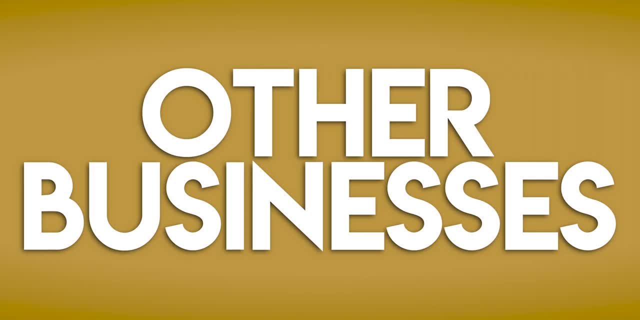 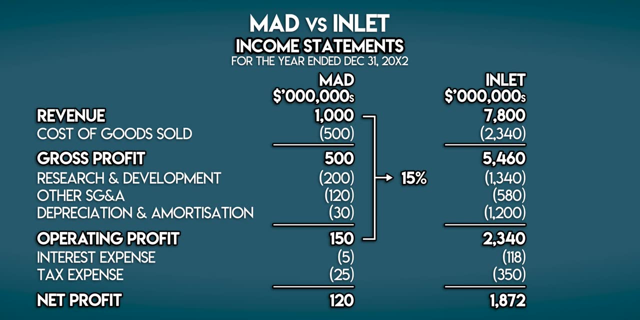 We can also compare operating profit margin against similar businesses. This time we've got the current year income statements for MAD and Inlet, two competitors in the same industry. Inlet is the market leader in semiconductor products and they earned a whopping $7.8 billion in revenue and their operating profit was. 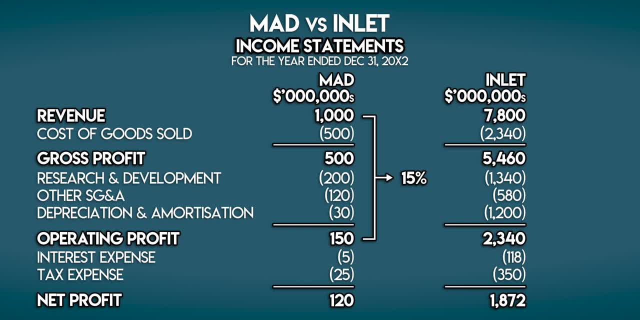 2.3% billion dollars. 2.34 divided by 7.8 is 0.3 or 30%. So not only is Inlet earning more revenue than MAD, they're also converting each dollar of that revenue into operating profits more. 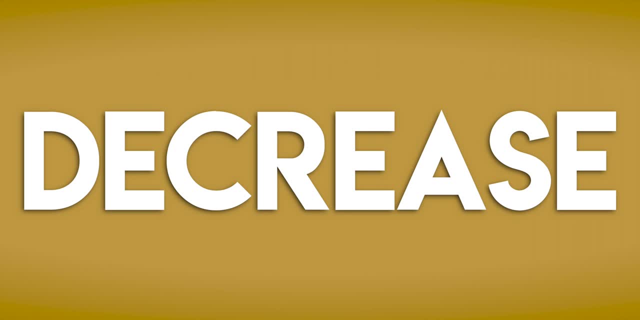 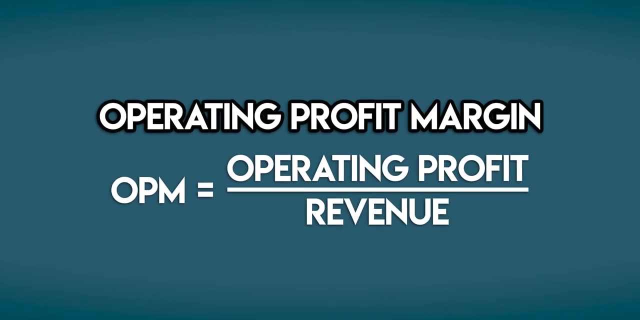 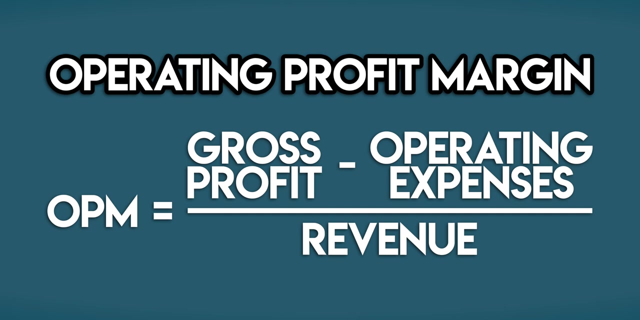 efficiently. What causes a decrease in operating profit margin Warning? I'm going to do a little bit of maths here to help explain this. Operating profit margin is operating profit divided by revenue. We saw earlier that operating profit is the same as gross profit minus operating expenses. 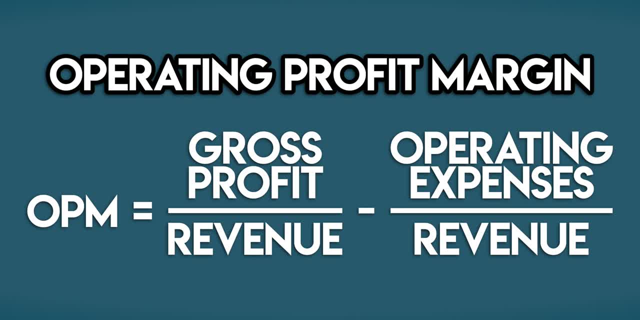 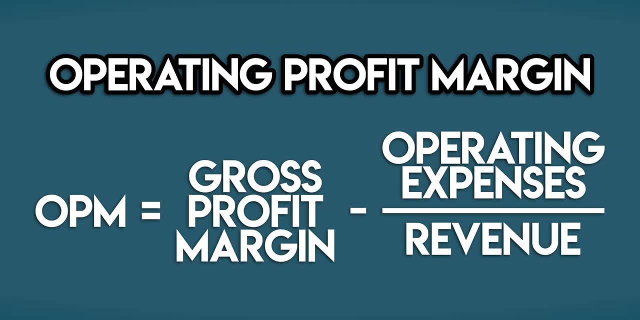 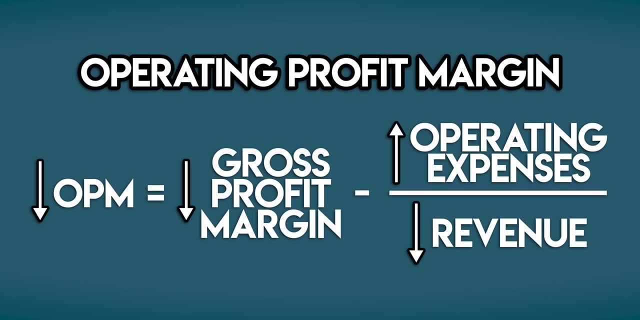 Now, if we separate this into two fractions and divide gross profit by revenue, then operating profit margin is equal to gross profit margin minus operating expenses divided by revenue. How does this help us? Well, it shows us that there are two ways that operating profit margin. 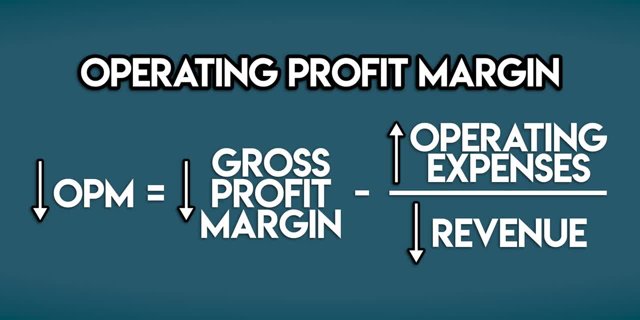 can decrease. Either the gross profit margin has gone down for all of the reasons mentioned in this video, or the operating profit margin has gone down for all of the reasons that I mentioned last time in the gross profit margin video, or operating expenses have increased as a proportion of revenue. Perhaps they're spending more on research and development. 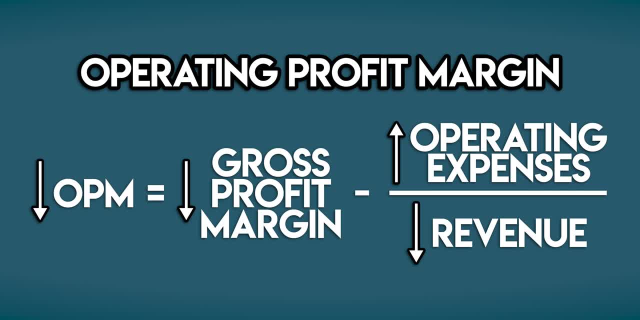 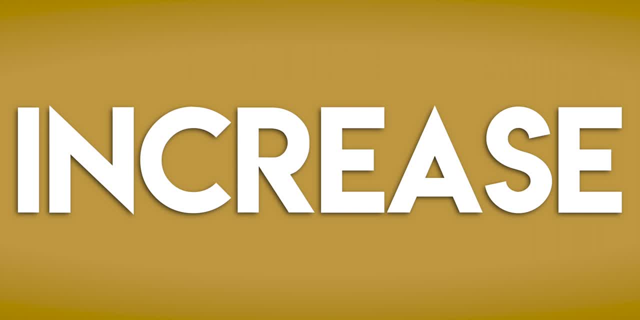 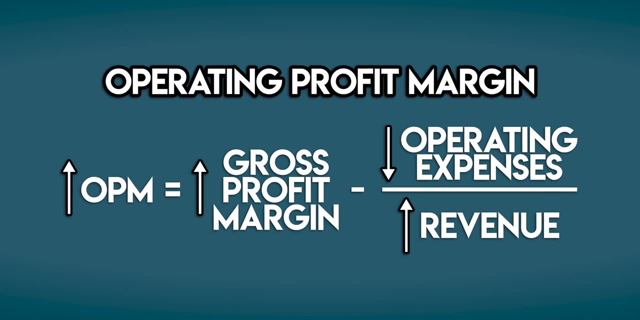 or administrative expenses, or maybe the business has been selling their products or services at a discount. On the other hand, what causes an increase in operating profit margin? We've still got the same formula, but the arrows are flipped around. Gross profit margin could have gone up. 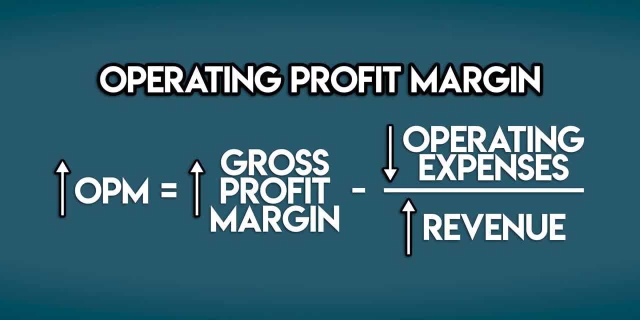 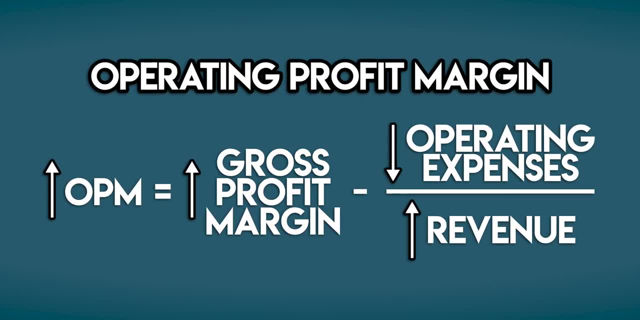 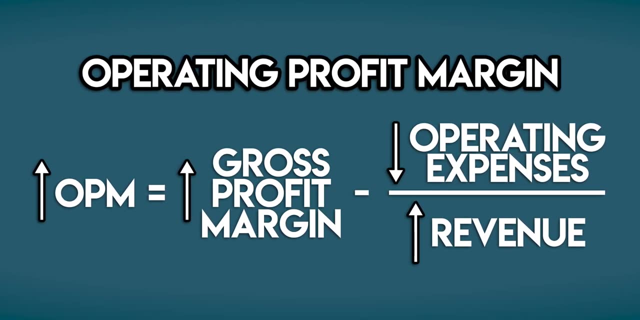 which would have a knock-on effect on operating profit margin, or the business's operating expenses have decreased relative to the revenue it earned, It could have hiked the prices on its products or services, or it could have reduced its operating expenses through better cost management. 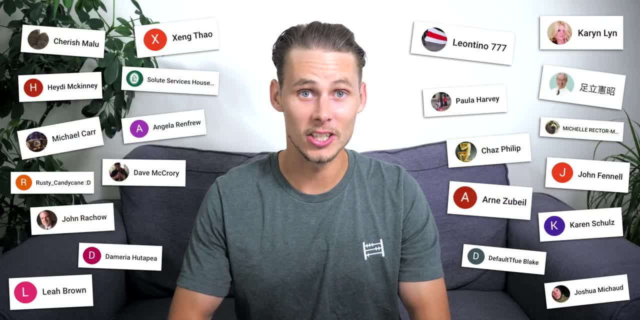 As always, a big thanks to all my channel members. Your donations help me make these accounting tutorials, so I value your support. Stay safe and I'll see you next time. 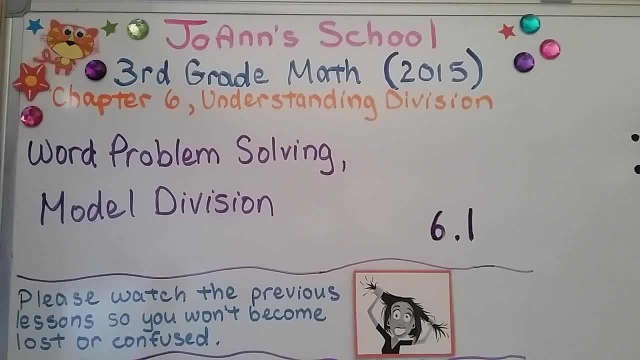 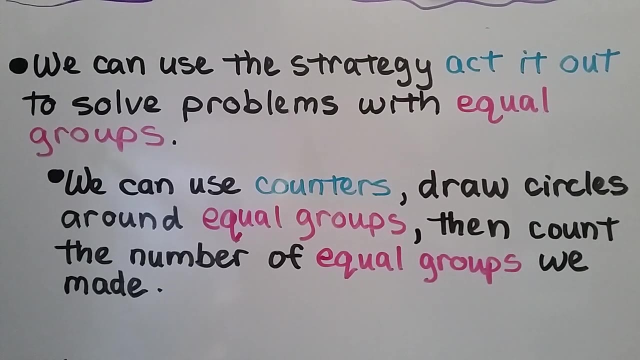 We're in a new chapter, chapter six, about understanding division. This is 6.1.. We're going to do word problem solving and model division with counters. We can use the strategy, act it out to solve problems with equal groups. We can use counters to draw circles around. 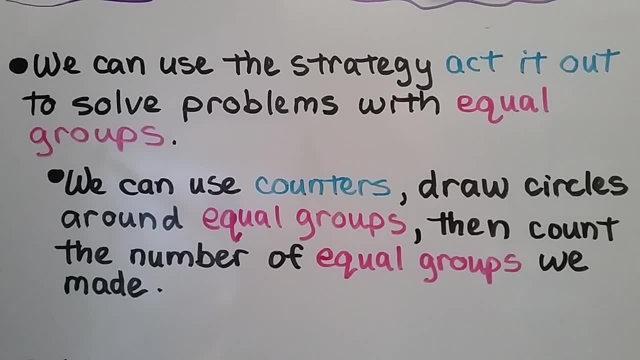 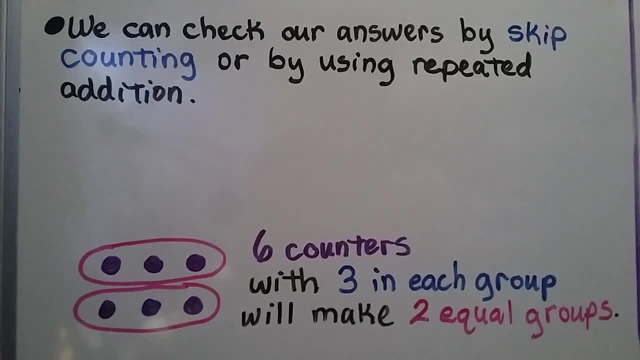 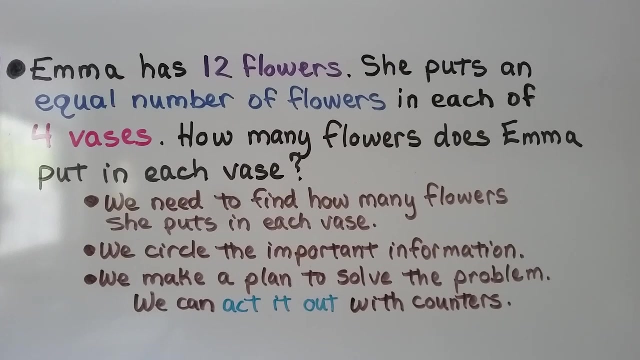 equal groups, then count the number of equal groups we made. We can check our answers by skip counting or by using repeated addition. Here we have six counters. with three in each group, It'll make two equal groups. Emma has 12 flowers. She puts an equal number of. 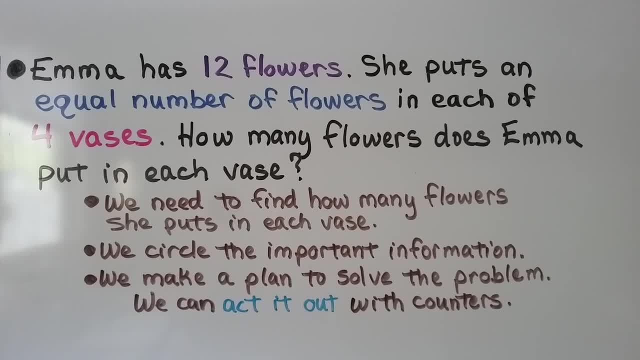 flowers in each of them. We have four vases. How many flowers does Emma put in each vase? We need to find how many flowers she puts in each vase. We circle the important information: There are 12 flowers and there are four vases, And she's going to put an equal number of flowers in each. 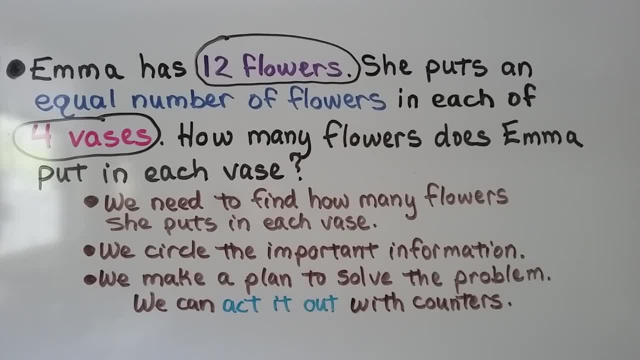 vase, isn't she? We make a plan to solve the problem. We can act it out with counters. We're going to do word problem solving and model division. We can use the strategy- act it out to solve problems with equal groups. We can use counters to draw circles around. equal groups. Here we have six counters with three in each group. We can use counters to draw circles around equal groups. Here we have six counters with three in each group. We can use counters to draw circles around equal groups. Here we have six counters with. three in each group. We can use counters to draw circles around equal groups. We can use counters to draw circles around equal groups. Here we have six counters, with three in each group. We can use counters to draw circles around equal groups. Here we have six counters.